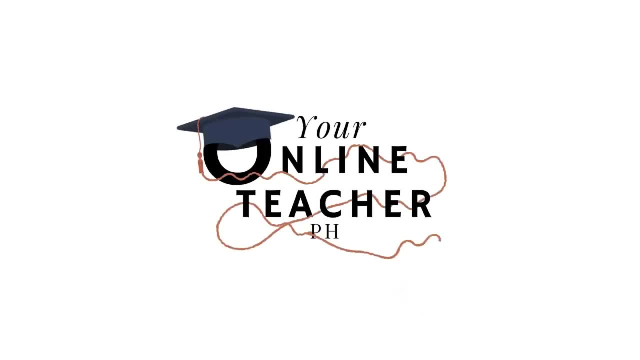 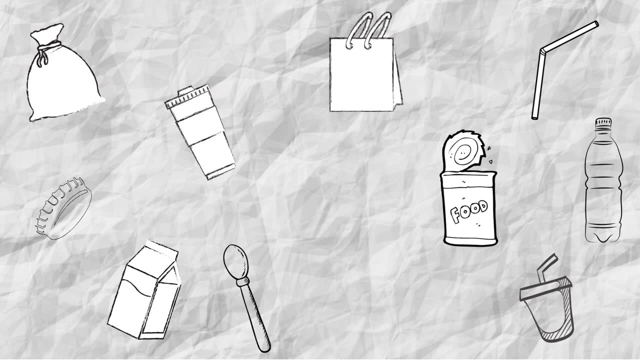 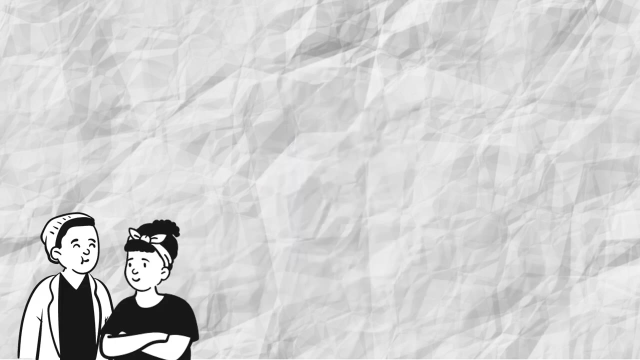 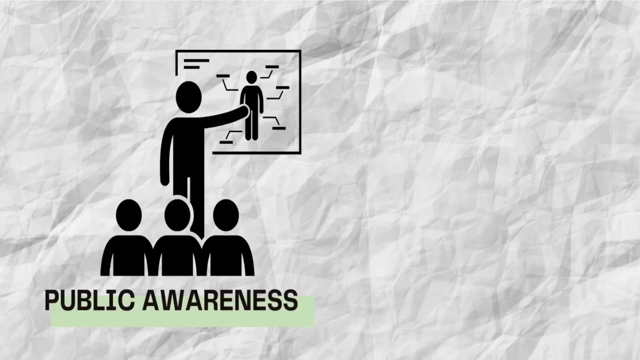 People use more and more convenient products because these can be easily disposed and replaced. This throwaway concept makes communities struggle with waste management problems. Everyone in the community is capable of making an impact on the solid waste problem through public awareness and action. Let us go and discover more about proper waste management. 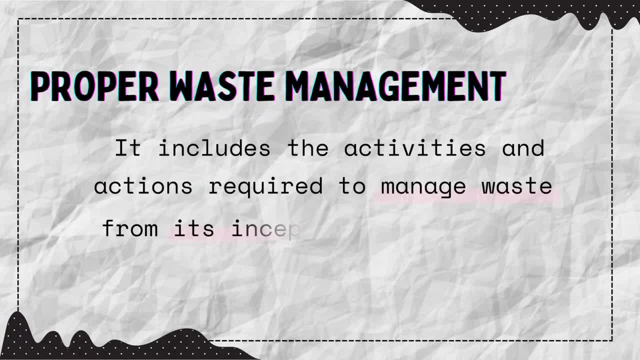 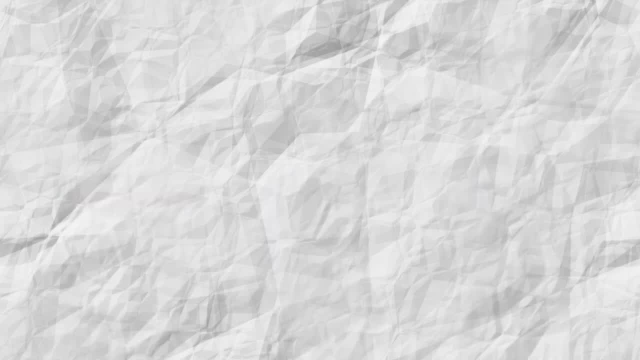 Proper waste management includes the activities and actions required to manage waste from its inception to its final disposal. Number one example is waste reduction. It can be done through reusing or finding other uses for objects. For example, instead of throwing your old clothes, give it to the less fortunate, or you can donate. 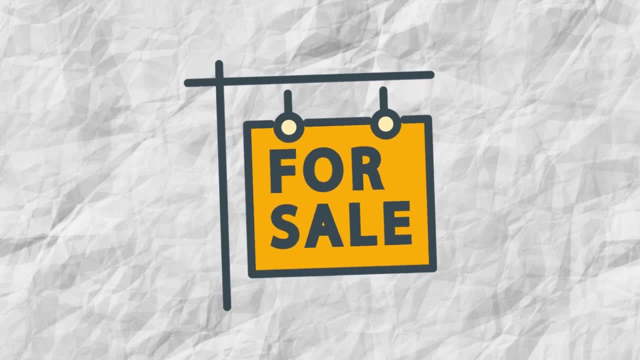 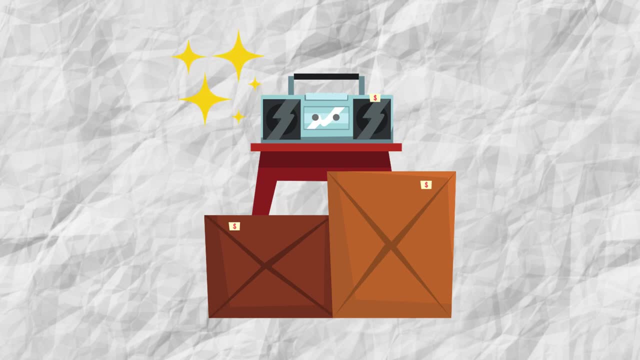 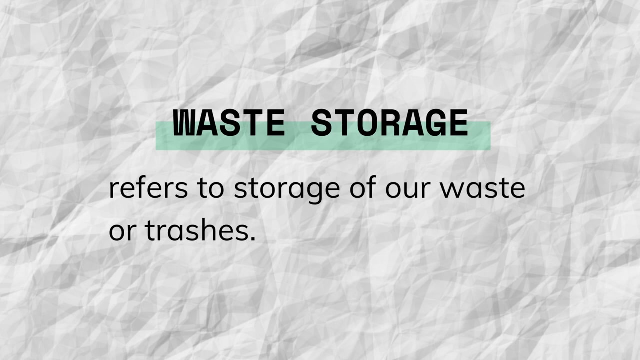 Garage sales are an opportunity to sell your unused or still functional items. Who knows, Your trash might be someone else's treasure. Unsold items can be donated to charity. Next is waste storage. Waste storage refers to storage of our waste or trashes. 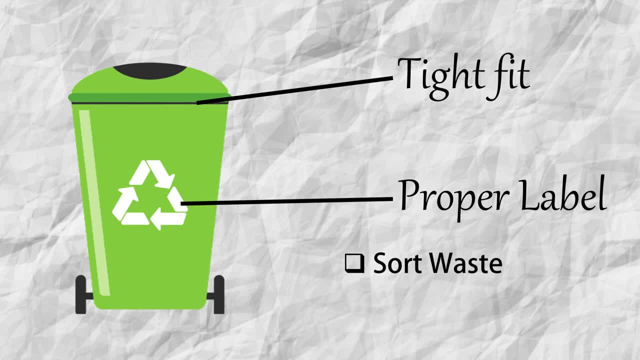